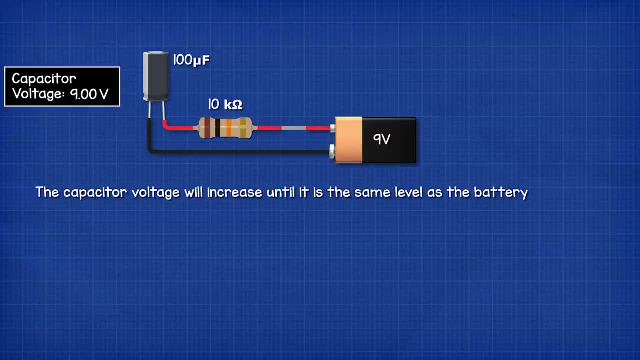 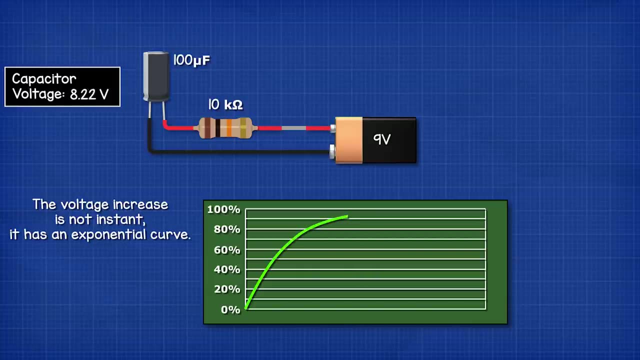 The voltage will increase until it is the same level as the battery. The voltage increase is not instant. It will have an exponential curve. At first the voltage increases rapidly and then it slows down until it reaches the same voltage level as the battery. We split this curve into six segments, but we're only interested in the 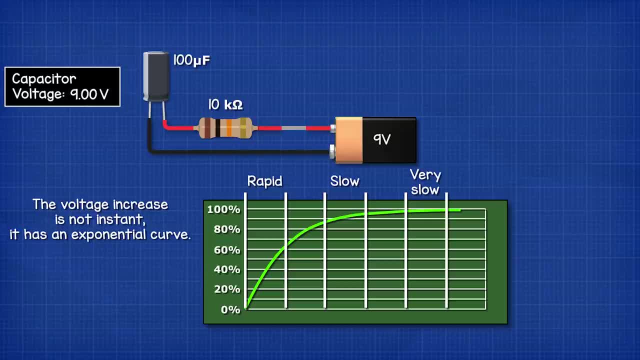 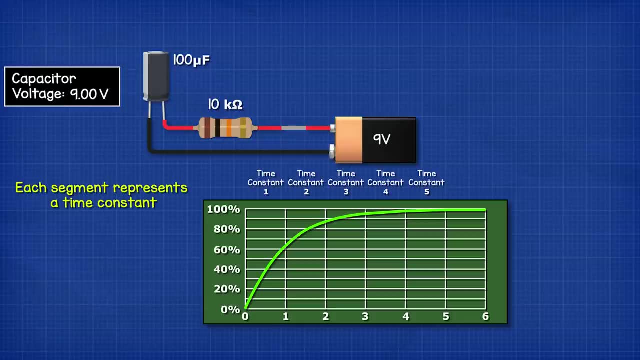 first five, because at the fifth marker we're basically at full voltage, so we can ignore anything past this. Each segment represents something called a time constant. Therefore, as we have five segments, we have five time constants, So it will take five time constants to charge the capacitor from zero. 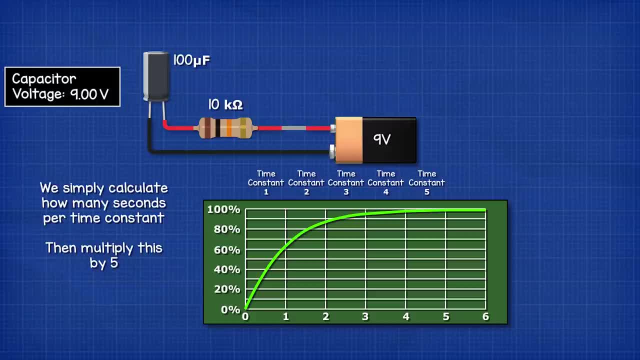 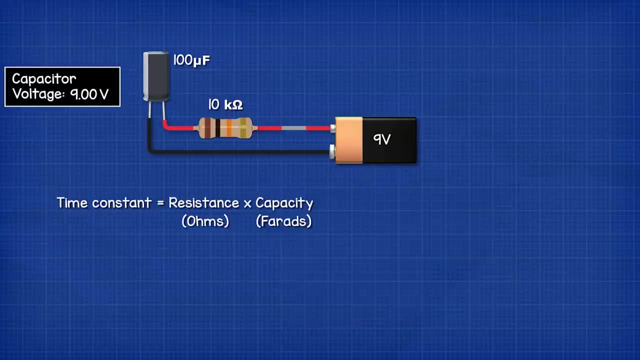 to just under 100 percent. All we need to do is to calculate how long one time constant is, and then we multiply this by five. To calculate the time constant we use this formula. Time constant in seconds equals the resistance in ohms multiplied by the capacity in farads. 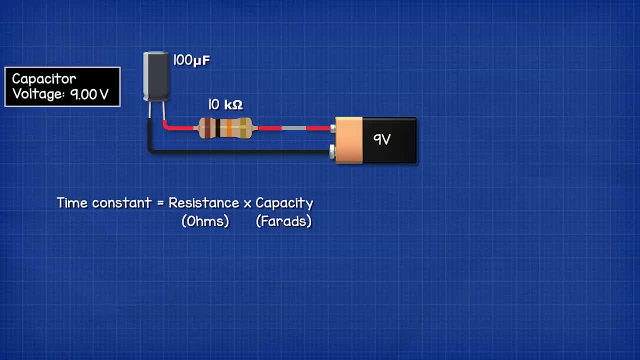 So we convert our resistor to ohms and our capacitor value to farads and we see that 10 000 ohms multiplied by 0.0001 farads equals 1.. So in this example, the time constant is equal to one second. Therefore, five of these is five seconds. 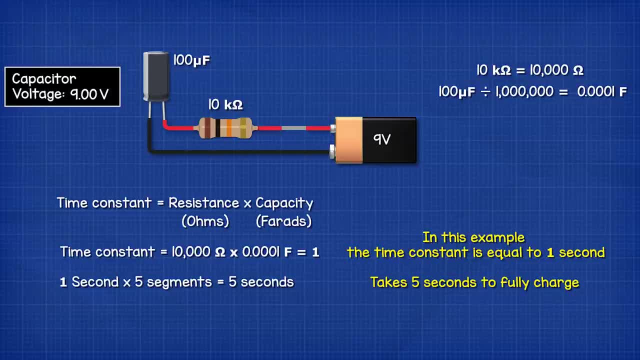 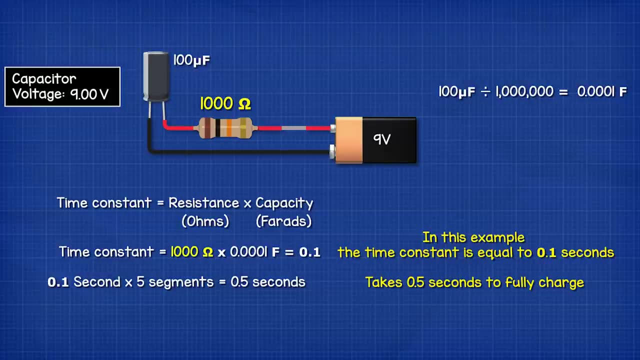 meaning it takes five seconds for the capacitor to fully charge to nine volts. If the resistor was just 1000 ohms, the time constant would be 0.1 seconds. so it would take 0.5 seconds to reach 9 volts. If the capacitor was 1000 microfarads, it would take 50 seconds in total. 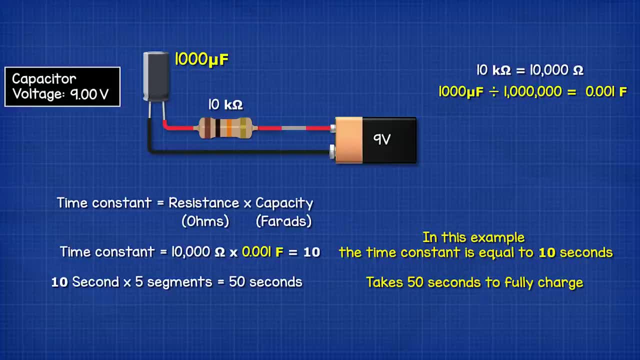 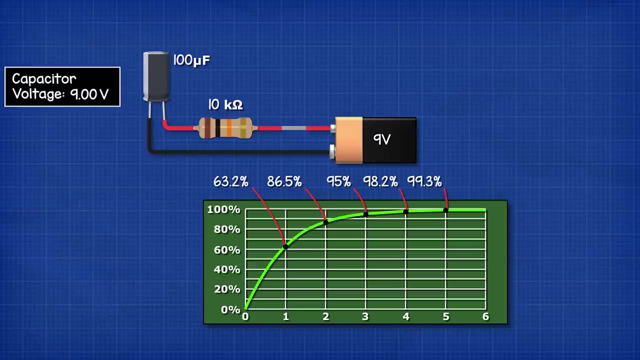 So as the capacitor size increases, the time taken will also increase. If the resistor value increases, then the time taken also increases. Coming back to our original circuit, we can therefore calculate the voltage level at each time constant. At 0.1 the voltage is always 63.2 percent, 0.2 is 86.5 percent, 0.3 is 95 percent. 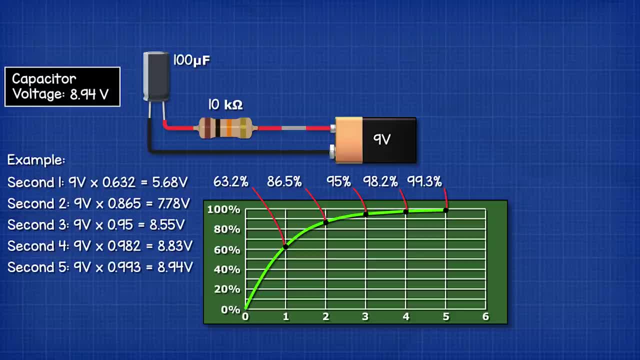 0.4 is 98.2 percent and 0.5 is 99.3 percent, So the voltage will never actually reach 100 percent. That's also why we stop at 0.1.. Now for some things. we can calculate the voltage level at just five points. 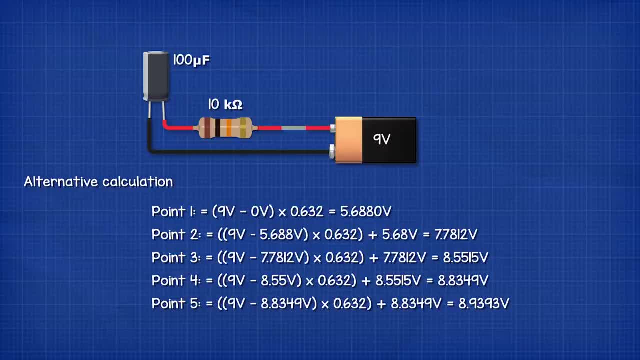 So in this example, after 1 second the capacitor voltage is 5.68 volts, After 2 seconds it's 7.78 volts, After 3 seconds it's 8.55 volts, After 4 seconds it's 8.83 volts, and after 5 seconds it's 8.94 volts. 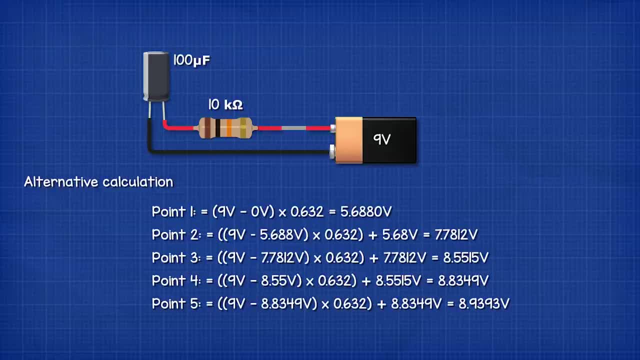 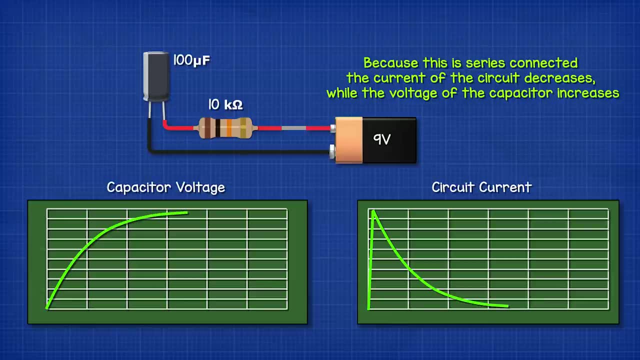 If you needed a more precise answer, we could also calculate each point like this: Remember: this voltage is always a constant, So it will always be the same voltage at any point of time, because this is in series. the current of the circuit decreases, while the voltage of the 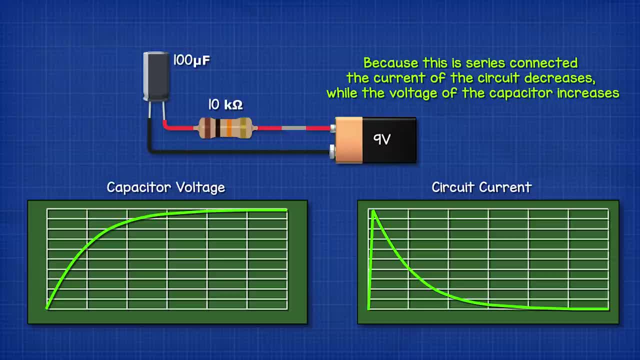 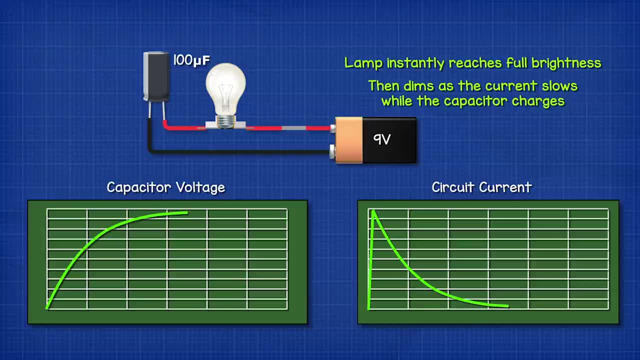 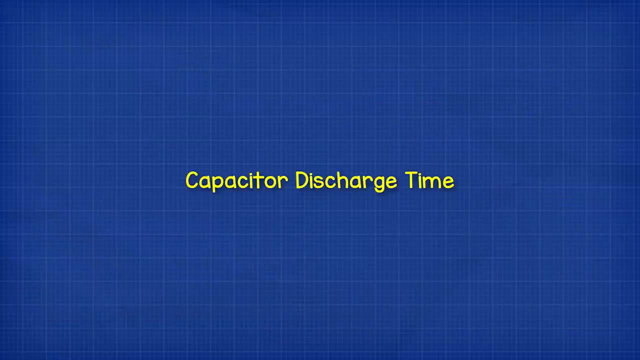 capacitor increases. Once at full voltage, no current will flow in the circuit. If the resistor was a lamp, it would therefore instantly reach full brightness when the switch was closed, but then becomes dimmer as the capacitor reaches full voltage. When we provide a path for the 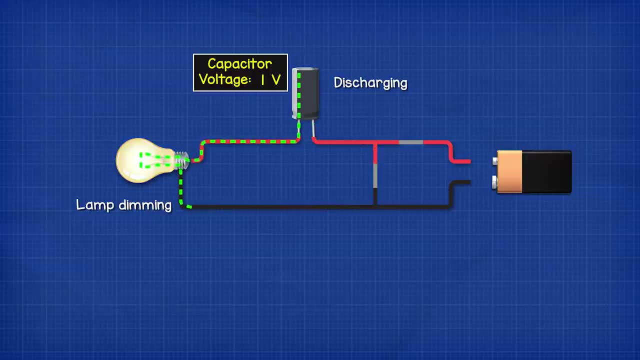 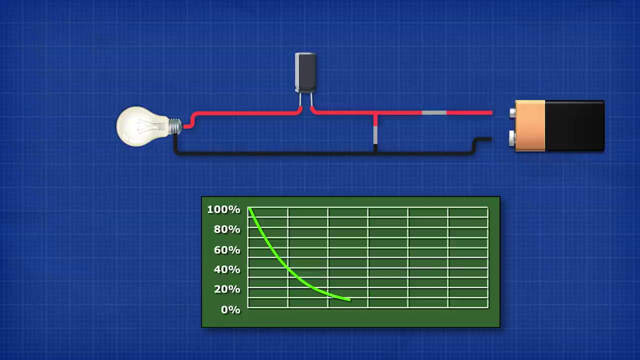 capacitor to discharge. the electrons will leave the capacitor and the voltage of the capacitor reduces. It doesn't discharge instantly but follows an exponential curve. We split this curve into six segments, but again we're only interested in the first five. At point one the voltage is always 36.8 percent. point two will be 13.5 percent. point three will be five percent. 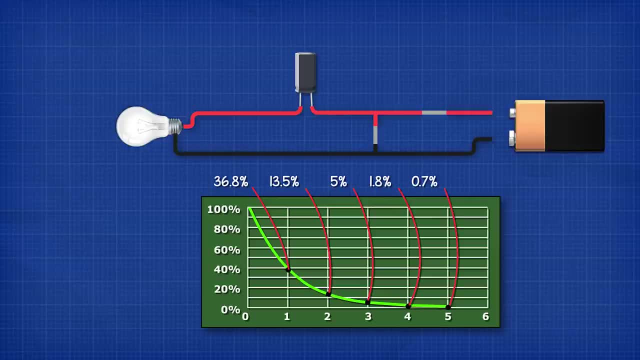 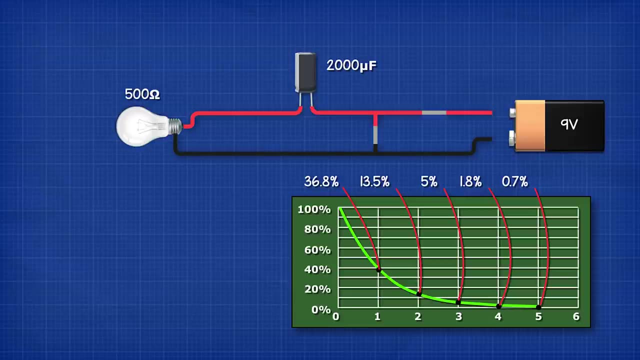 point four will be five percent will be 1.8% and 0.5 will be 0.7%. For example, if we had a 9-volt battery, a lamp with a resistance of 500 ohms and a 2000 microfarad capacitor, our time constant would be 500 ohms multiplied by 0.002.